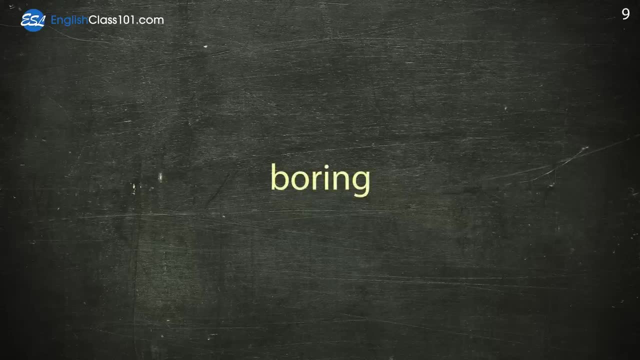 boring, boring, bright, bright, busy, busy, calm, calm, cheap, cheap, clean, clean, cloudy, cloudy, cold, cold, cool, cool, cute, cute, dark, dark, delicious, delicious, different, different, difficult, difficult, dirty, dirty, disgusting, disgusting, dissatisfied, dissatisfied. 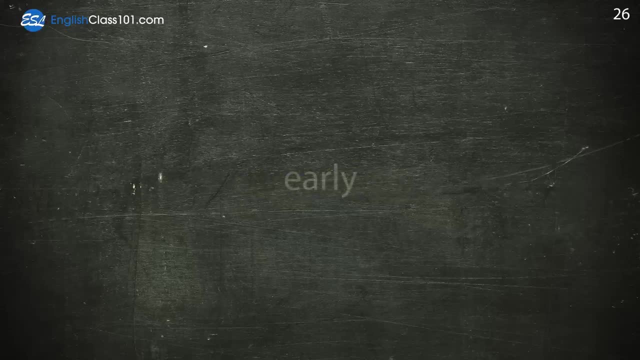 early, early, easy, easy, embarrassed, embarrassed, embarrassed, embarrassed, excited, excited, exciting, exciting, expensive, expensive, famous, famous, famous, famous, far foreign, free, fool, funny, good, great, great, happy, happy, hard, hard, heavy, heavy, high, high. 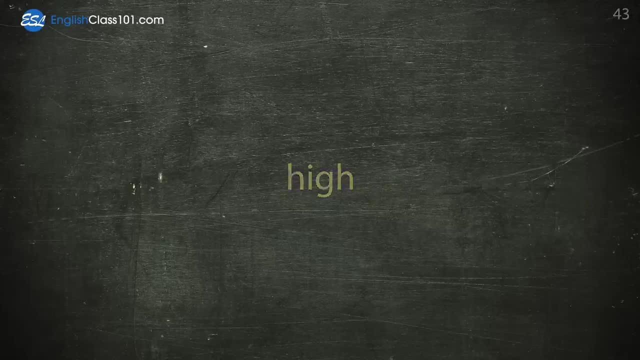 hot, hot, humid, humid, hungry, hungry, important, important, intelligent, intelligent, interesting, interesting, kind, kind, large, large, late, late, light, light, lively, lively, long, long, loud, loud, low, low, married, married mean mean narrow, narrow, near, near. 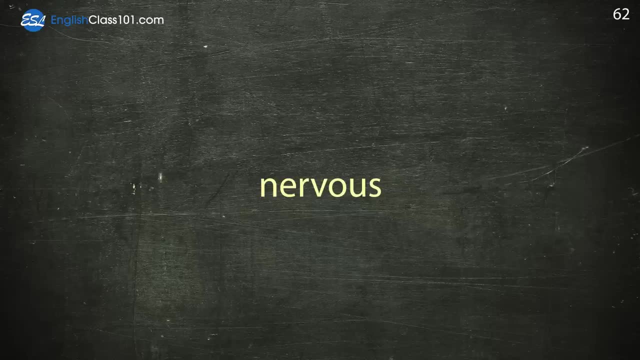 nervous, nervous, new, new, nice, nice, old, old, painful, painful, poor, poor, poor, poor, poor, painful, painful, quiet, quiet, quiet, quiet, rainy, rainy, relaxing, relaxing, rich, rich, rich, rich, happy, rich, happy, rich, right old. 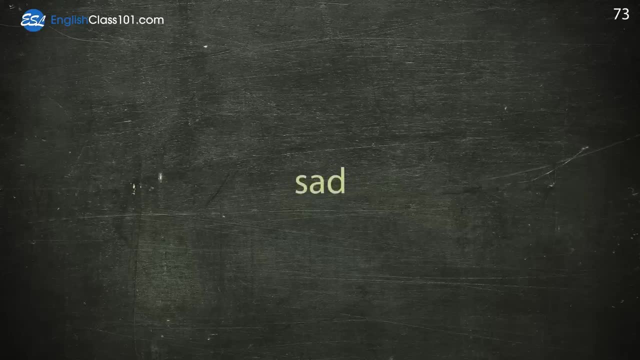 old, old, bright, bright, sad, sad, sad, sad, sad, sad, salty, salty, salty, salty. same same, same same. satisfied, satisfied, Satisfied. Scary, Scary, Serious, Serious, Short Short, Shy, Shy. 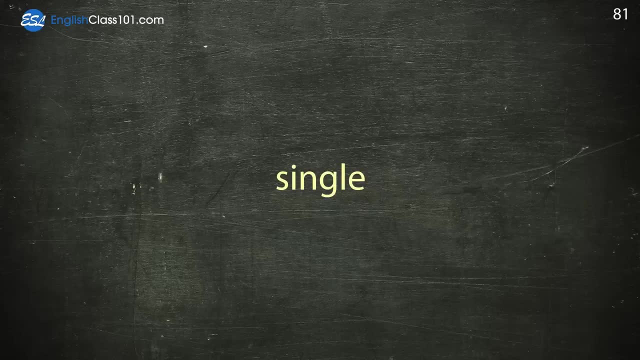 Single, Single, Small, Small, Soft, Soft, Sour, Sour, Special, Special Spicy, Spicy, Strong, Strong, Sunny, Sunny, Sure, Sure, Sure, Sweet, Sweet, Tall, Tall Thirsty. 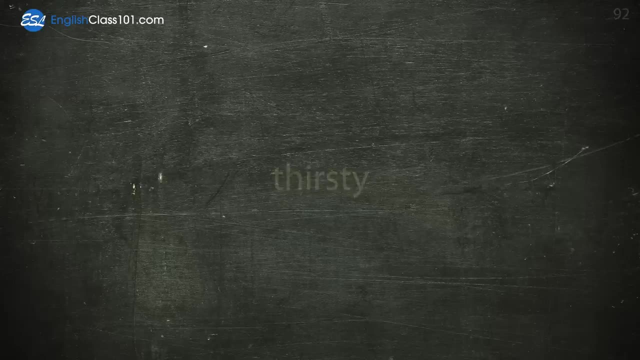 Thirsty, Tired, Tired, Tired, True, True, Ugly, Ugly, Ugly, Warm, Warm, Weak, Weak, Wide, Wide, Windy, Windy, Dulce Saudia Sweet. 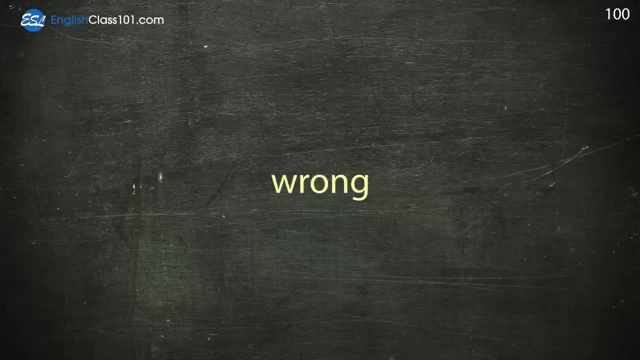 Fervently 걸고: Tremble, Windy, Terrible, Math, Malード yscy Right Windy, Receive Fine, Stress, Unbelievable, Accusative, melancholic Because of selling books. Consistent Unrighteousness, Repentance Manied Being late F 절�edmerelo graphicolo T 소� suburban newspaper, Unlikely To not know about the excuses. Young, Young, Novoclad regul.